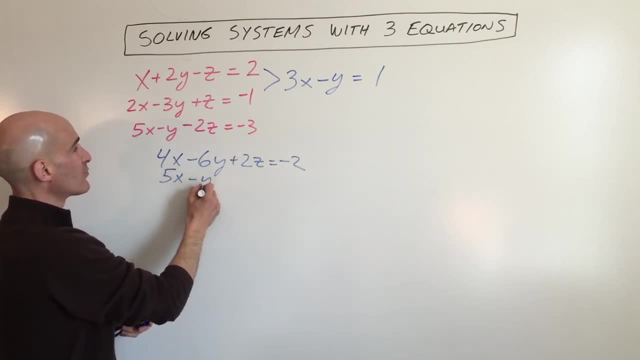 4z equals negative 2.. The third equation I'm just going to bring down, and we're going to add these two together. So if we do that, we get 9x minus 7y equals negative 5.. Okay, now we're down. 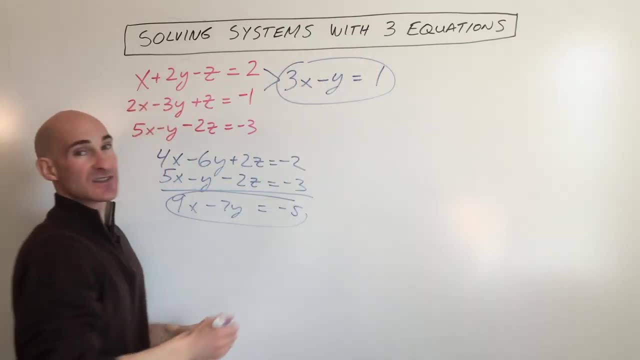 to two equations with two variables, just x's and y's. So let's multiply this equation by negative 7, so we get a positive 7y. We can add it to this equation and eliminate the y's, So if we do that, we get 21x. 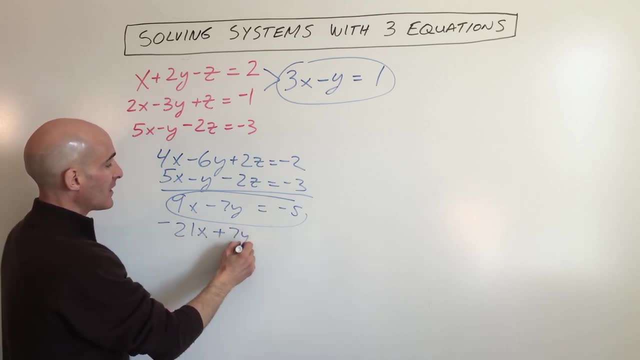 Okay, negative 21x plus 7y equals negative 7.. We're going to add those together: We get negative 12x. The y's cancel, We get negative 12.. Divide by negative 12. x equals 1.. So we went. 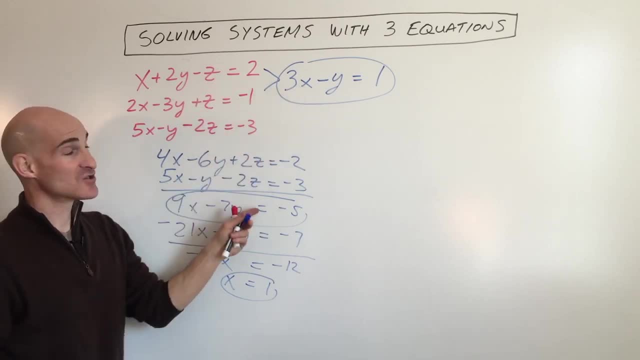 from three equations with three variables down to two equations with two variables, down to one equation with one variable. Now we're going to work our way backwards, Okay, so we're going to put this into one of the equations that has just two variables. Let's put it into this one over. 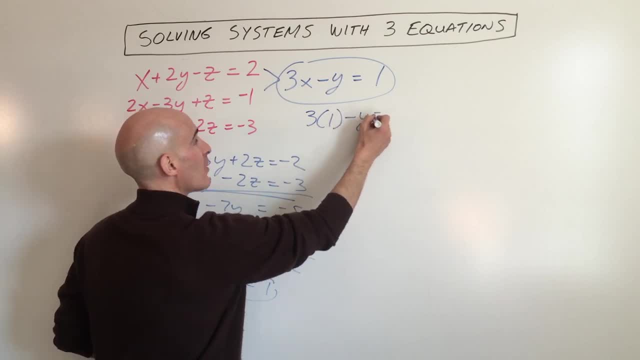 here. So 3 times 1 minus y equals 1. We put in 1 for x. So subtract 3 from both sides, That gives you negative 2.. Divide by negative: 1. y equals 2.. So now we know what x and y are. Let's go ahead and 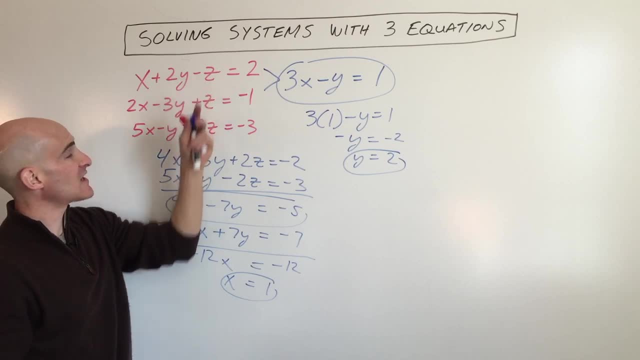 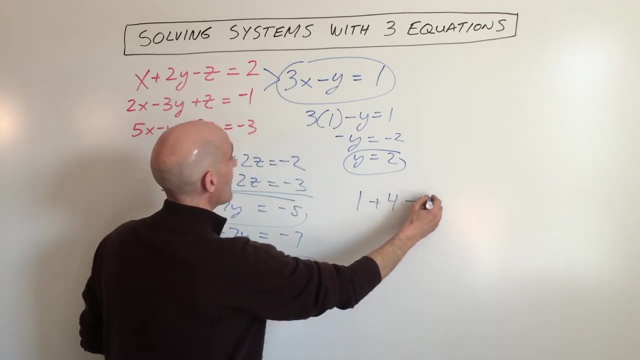 put it back into one of the original equations to solve for z. So we'll just do this top one. So we have: 1 plus y is 2.. So 2 times 2 is 4 minus z equals 2.. That's 5 minus z equals 2.. So that's. 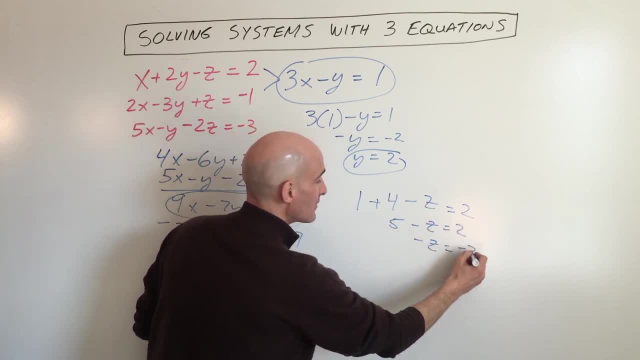 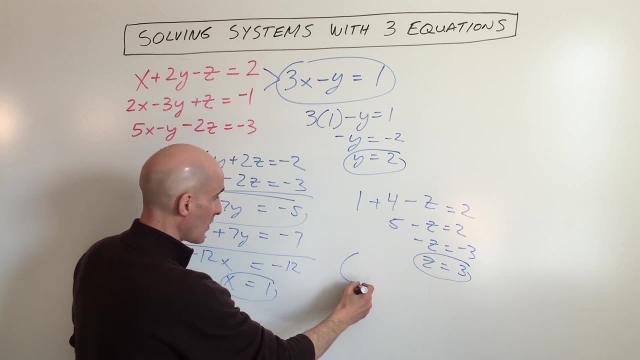 5 minus z equals 2.. Subtract: 5. That equals negative. 3. Divide by negative: 1. z equals 3.. So now we have x, y and z And we're going to write this as a triple: x, y, z. Alphabetical order: 1,, 2, 3. x, y, z. Okay, so you just write it as a triple.